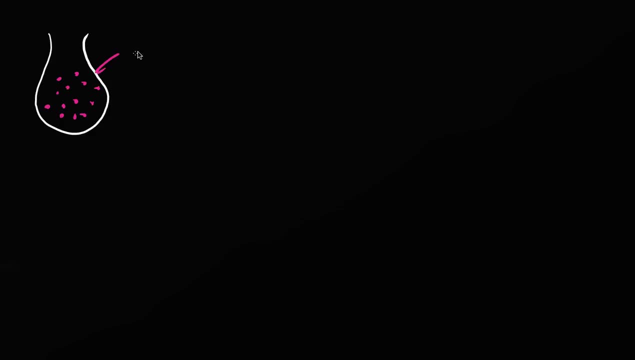 I'm not gonna draw all of them, but you get the general idea. There are going to be 50 magenta marbles, 15 magenta marbles And there's also going to be 50 blue marbles. So 50, 50 blue marbles. 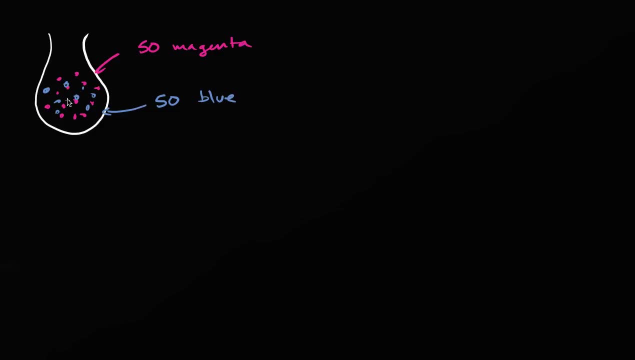 And what you do is you have these 100 marbles in there- half of them magenta, half of them blue- and before picking a marble out- and you're gonna be blindfolded when you pick a marble out- you shake the bag. 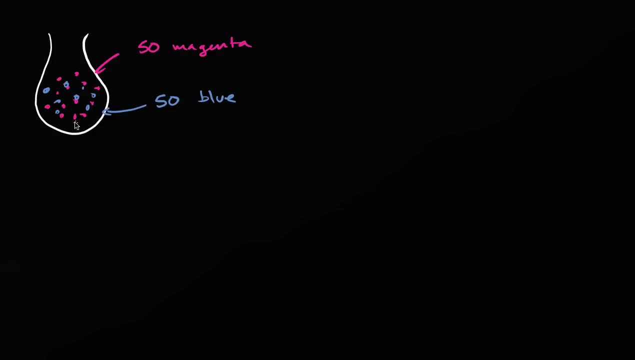 You shake the bag really good to, so you think, mix them up a little bit. And so if you were to say, well, theoretically, what is the probability if you stuck your hand in and you're not looking, what is the probability of picking? 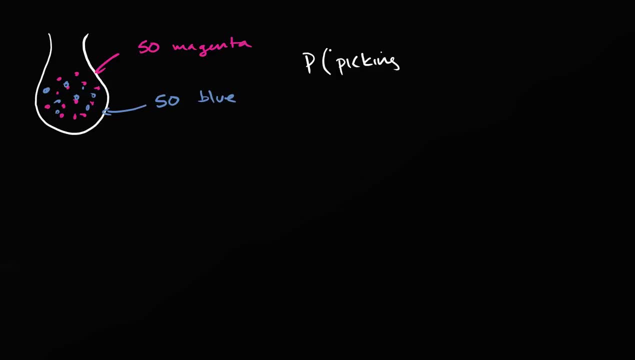 of picking a magenta. I have to feel the need to write the word magenta in magenta. What is the probability of picking a magenta marble? Well, theoretically, there's 100 equally likely possibilities. There's 100 marbles in the bag. 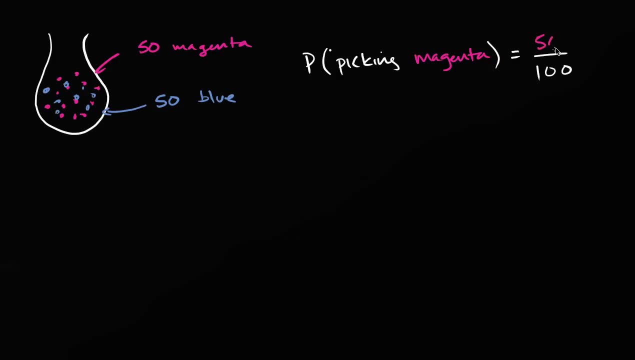 And 50 of them involve picking a magenta. So 50 out of 100, and this is the same thing as a 1 1⁄2 probability. So you could say, well, theoretically, 50 out of 100, and this is the same thing as a 1 1⁄2 probability. So you could say, well, theoretically, 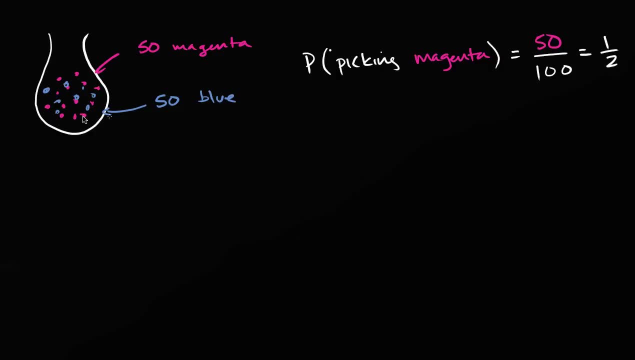 there is a 1 1⁄2 probability. I just did the math. If you say these are 100 equally likely possibilities, 50 of them are picking magenta. Now let's say you actually start doing the experiment, So you literally take a bag with 50 magenta marbles. 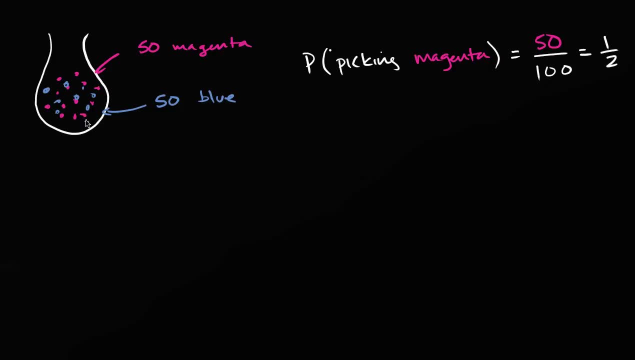 50 blue marbles and then you start picking. you start picking the marbles and then you see what marble color you picked and you put it back in and then you do it again. And so let's say that after 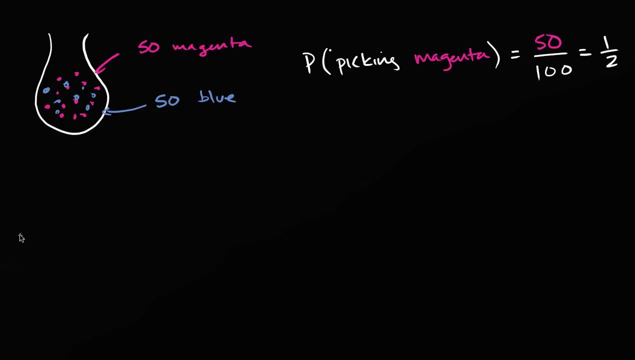 let's say that after every time you put your hand in the bag and you take something out of the bag and you observe what it is, we're gonna call that an experiment. So, after, after 10 experiments, 10 experiments, after 10 experiments. 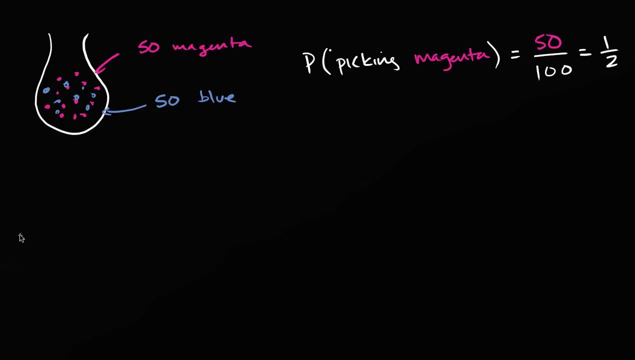 let's say that after every time you put your hand in the bag and you take something out of the bag and you observe what it is, we're gonna call that an experiment. So, after, after 10 experiments, 10 experiments, after 10 experiments. 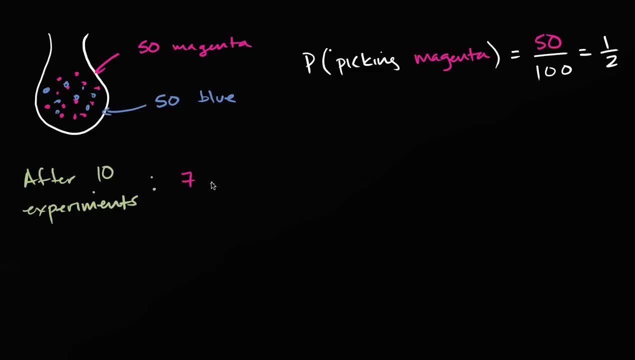 let's say that you have picked out seven magenta, seven magenta and three blue and three blue. So does this cause, is this strange, that after 10, out of the first 10 experiments, you haven't picked out exactly half of them being magenta? 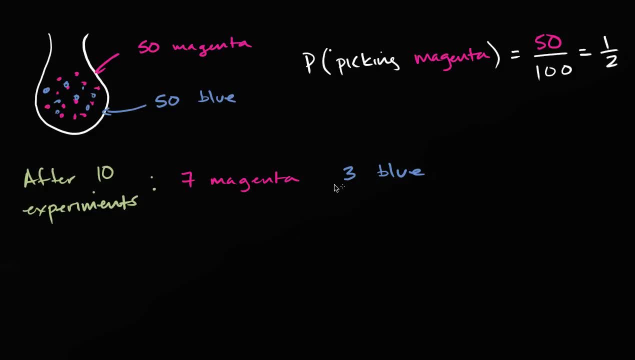 You've picked out seven magenta and then the other three were blue. Well, no, this is definitely a reasonable thing. If the true probability of picking out a magenta is 1 1⁄2,, it's definitely possible that you could still pick out seven magenta. 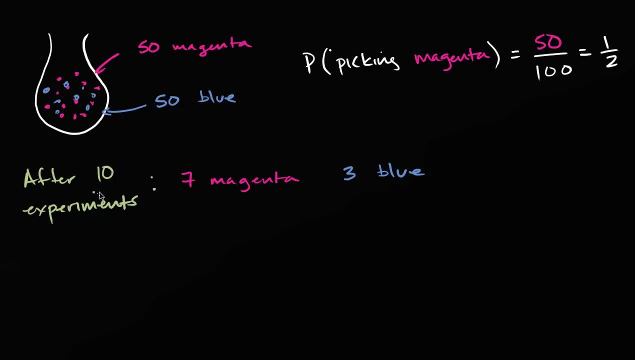 Did that just happen to be what your fingers touched? And this isn't a lot of experiments. It's completely reasonable that out of 10, yeah, you could have a, and you know, later on in statistics we'll define these things in more detail. 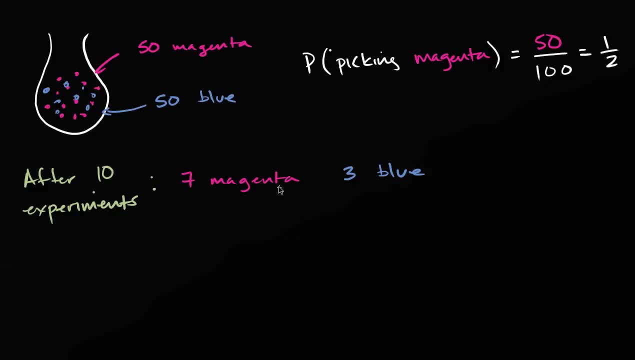 but there's enough variation in where you might pick that you're not going to always get, especially with only 10 experiments. you're not definitely going to get exactly 1⁄2.. You can, you know, instead of having five magenta. 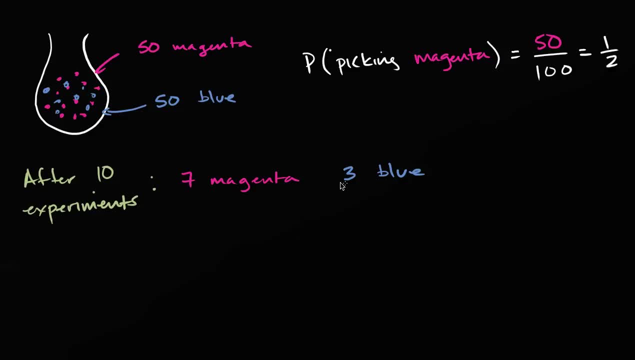 it's completely reasonable to have seven magenta, So this really wouldn't cause me a lot of pause. I still wouldn't say hey, I still wouldn't question what I did here when I calculated this theoretical probability. But let's say: 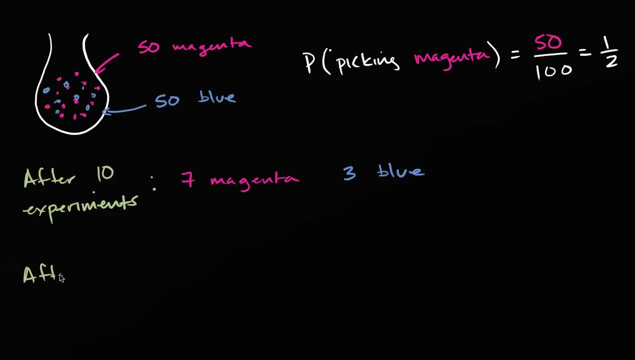 and let's say you have a lot of time on your hands. and let's say after, let's say after 10,000 trials here, after 10,000 experiments- and remember the experiment, you're sticking your hand in the bag- 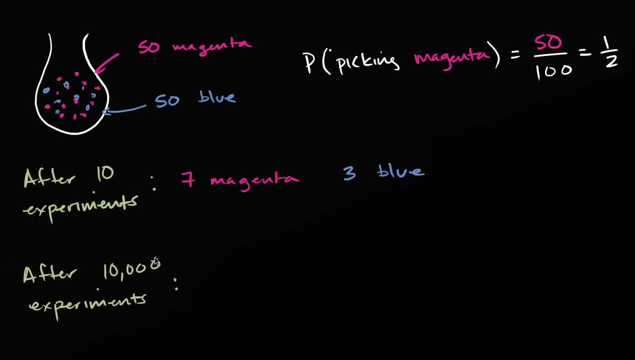 without looking with your fingers, kind of feeling- around, picks out a marble and you observe the marble and you record what you found. And so let's say, after 10,000 experiments you get seven 7,000, 7,000 magenta. 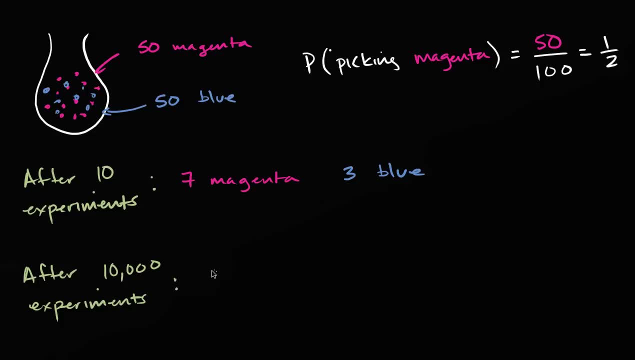 Actually, let me do slightly different numbers. Actually, let me make it even more extreme. Let's say: you get 8,000, 8,000 magenta and you have 2,000 blue, 2,000, 2,000 blue. 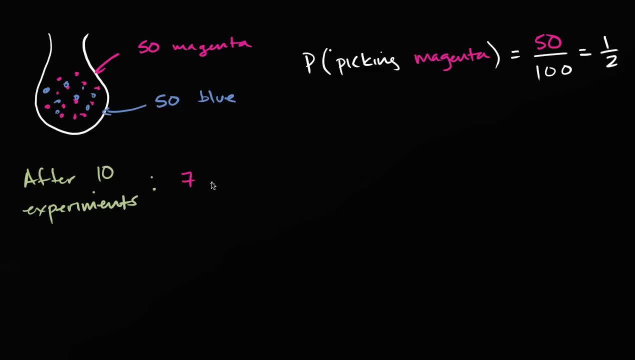 let's say that you have picked out seven magenta, seven magenta and three blue and three blue. So does this cause, is this strange, that after 10, out of the first 10 experiments, you haven't picked out exactly half of them being magenta? 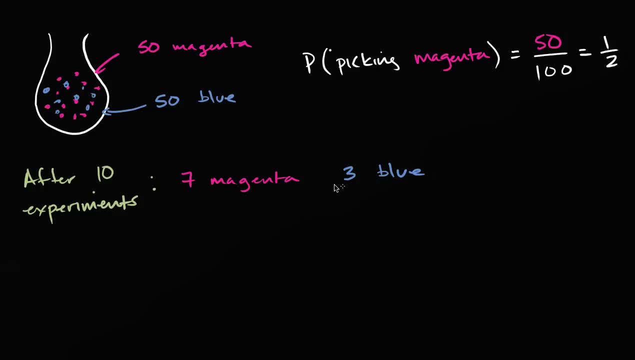 You've picked out seven magenta and then the other three were blue. Well, no, this is definitely a reasonable thing. If the true probability of picking out a magenta is 1 1⁄2,, it's definitely possible that you could still pick out. 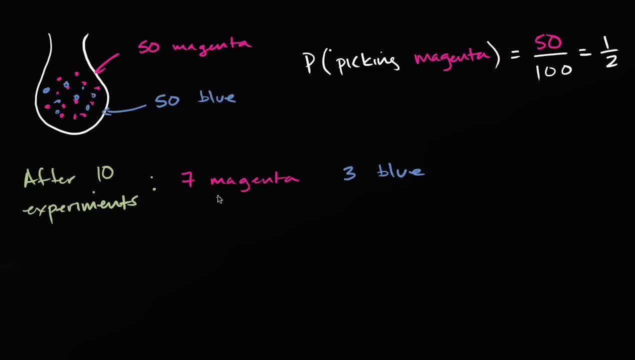 seven magenta. That just happened to be what your fingers touched And this isn't a lot of experiments. It's completely reasonable that out of 10, yeah, you could have a, and you know, later on in statistics we'll define these things in more detail. 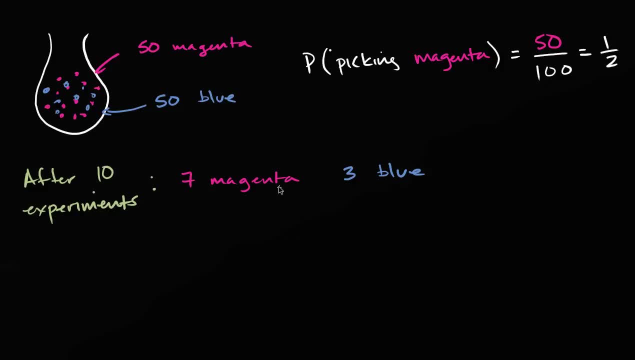 but there's enough variation in where you might pick that you're not going to always get, especially with only 10 experiments. you're not definitely going to get exactly 1⁄2.. You can, you know, instead of having five magenta. 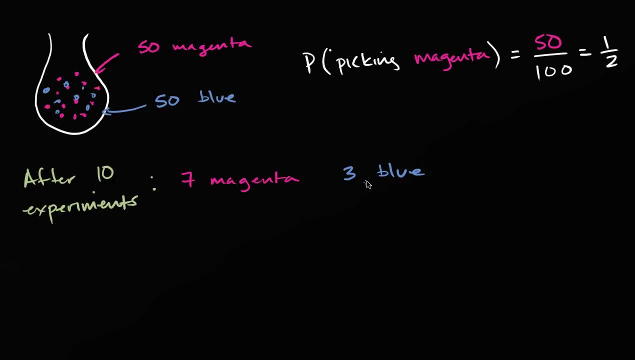 it's completely reasonable to have seven magenta. So this really wouldn't cause me a lot of pause. I still wouldn't say hey, I still wouldn't question what I did here when I calculated this theoretical probability. But let's say, and let's say, you have a lot of time. 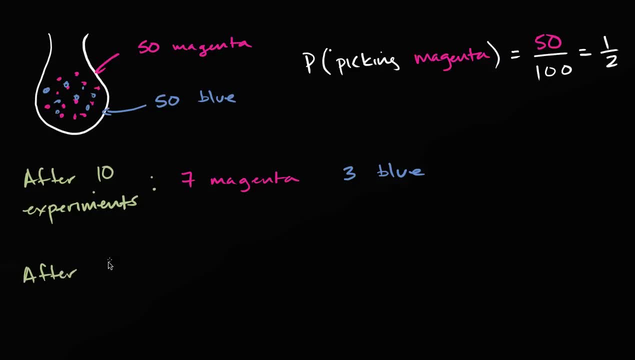 on your hands and let's say after, let's say after 10,000 trials here, after 10,000 experiments, and remember the experiment. you're sticking your hand in the bag without looking with your fingers, kind of feeling around. 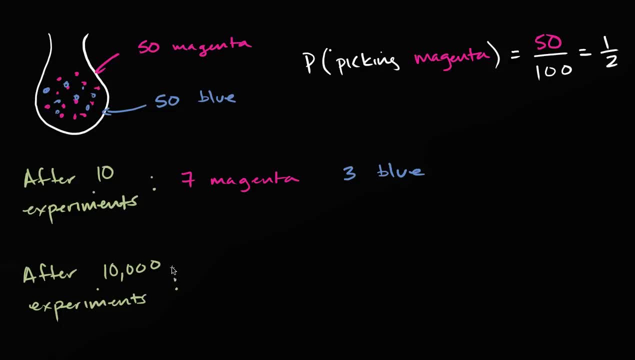 picks out a marble and you observe the marble and you record what you found. And so let's say, after 10,000 experiments you get 7,000, 7,000 magenta. Actually, let me do slightly different numbers. 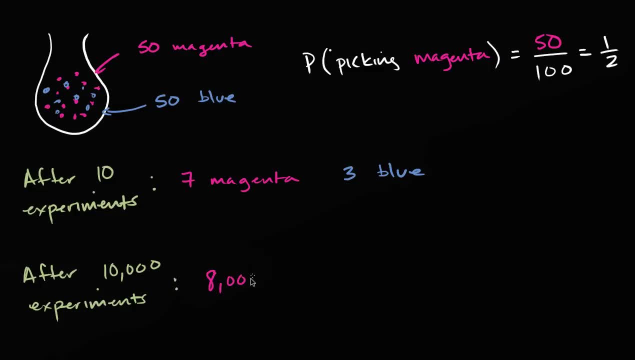 Actually, let me make it even more extreme. Let's say: you get 8,000, 8,000 magenta and you have 2,000 blue, 2,000, 2,000 blue. Now this is interesting because here 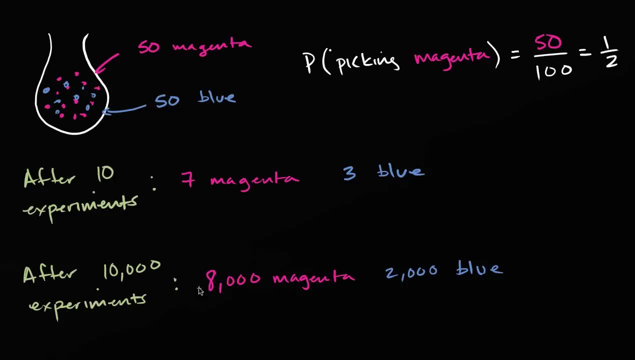 Now this is interesting because here what you're seeing experimentally seems to be very different, and now you have a large number of trials right Right over here, Not just 10.. 10 is completely reasonable That. hey, you know, I got seven magenta. 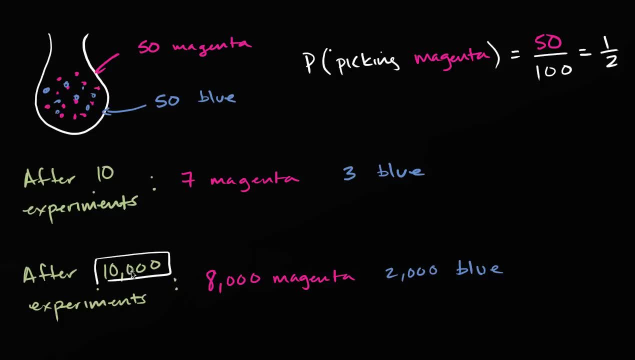 and three blue instead of five and five. But now you've done 10,000.. 10,000.. And it's definitely you know you would have expected, if this was the true probability, you would have expected that half of these. 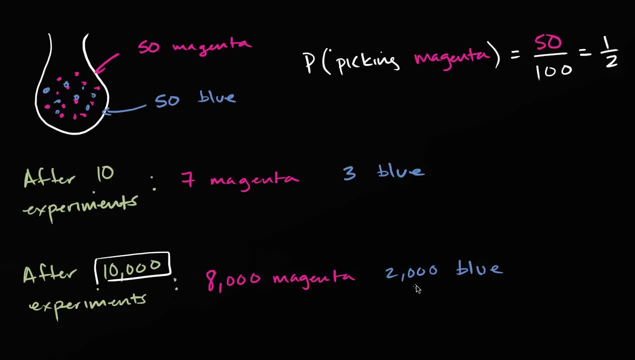 would have been magenta, Only 5,000 magenta and 5,000 blue, But you had 8,000 magenta. Now, this is within the realm of possibility if the true probability of picking a magenta is one half. 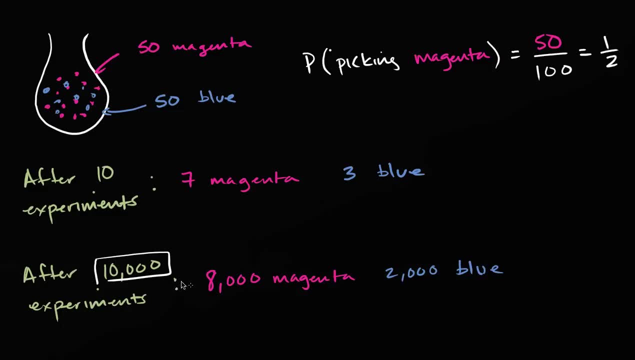 but it's not. it's very unlikely that you would have gotten this result with this many experiments, this many trials. if the true probability is one half, Here your experimental probability, your experimental probability is showing. look out of 10,000 trials. 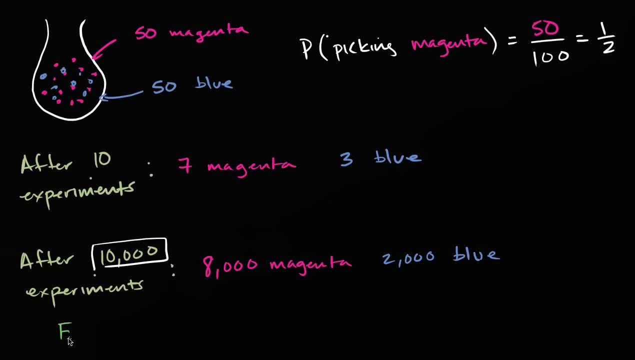 actually let me write that here: experimental probability. experimental probability here is: you had 10,000 trials and or 10,000 experiments, I guess you could say, and you, and in 8,000 of them you got a magenta marble. 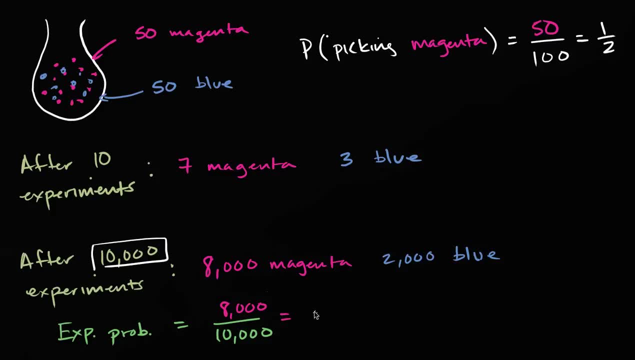 And so this is going to be 80%, or eight tenths, So 80%. So there seems to be a difference here, And the reason why I would take this more seriously is that you had a lot of trials here. You did this 10,000 times. 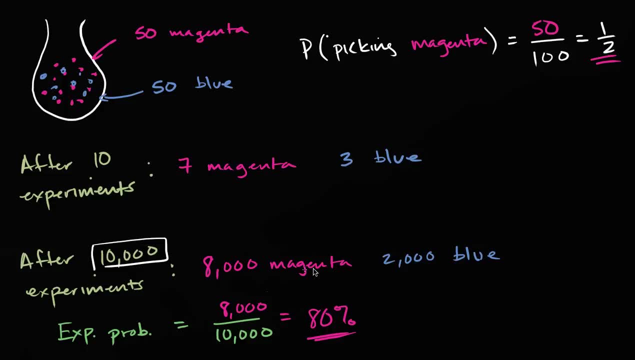 If the true probability was one half, it's very low likelihood that you would have gotten this many magenta. So when you think about it, you're like: look well, what, what did I? what's going on here? What are possible explanations for this? 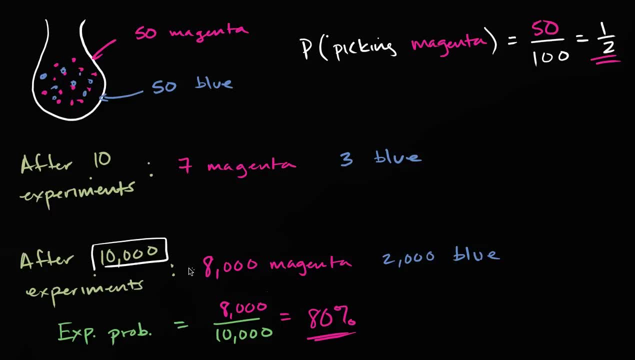 This I wouldn't have fretted about. After 10 experiments- not a big deal, But after 10,000, this would have caused me pause. Say well, why would this happen? I mixed up the bag every time And there's some different possibilities. 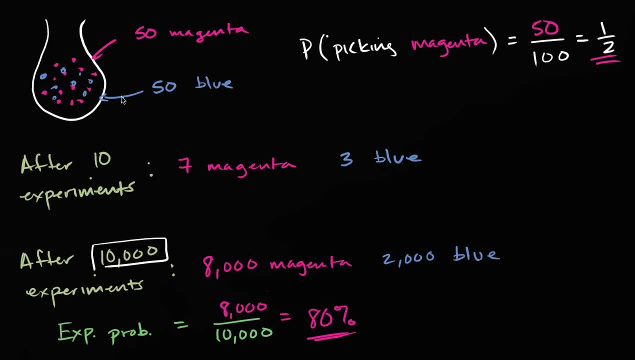 Maybe the blue marbles are slightly heavier, and so when you shake the bag up enough, the blue marbles settle to the bottom and you're more likely to pick a magenta marble. Maybe the blue marbles have a slightly different texture to them. 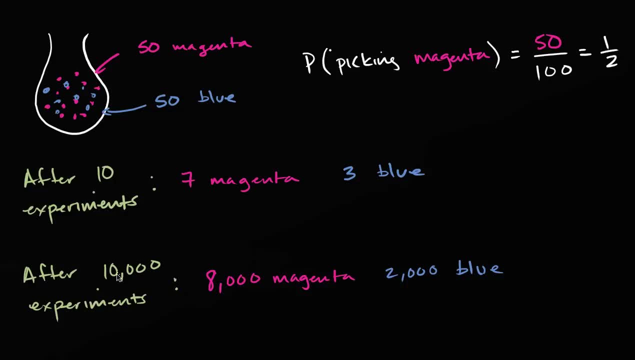 what you're seeing experimentally seems to be very different. And now you have a large number of trials right over here, Not just 10.. 10 is completely reasonable, That, hey, you know. I got 7 magenta and 3 blue. 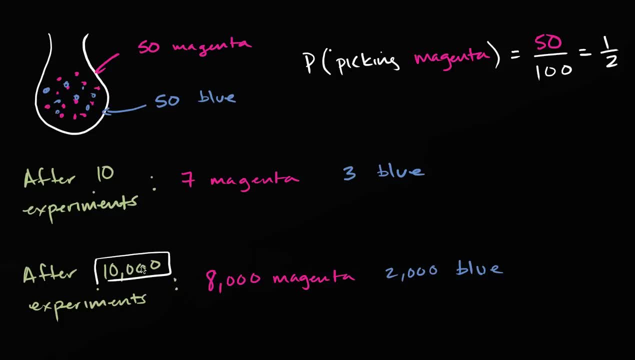 instead of 5 and 5.. But now you've done 10,000.. 10,000.. And it's definitely you know you would have expected, if this was the true probability, you would have expected that half of these. 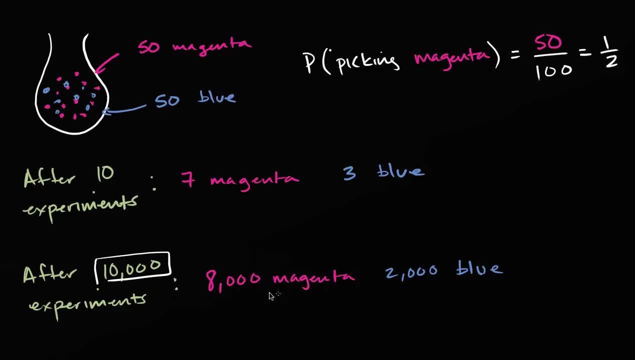 would have been magenta, Only 5,000 magenta and 5,000 blue, But you had 8,000 magenta. Now, this is within the realm of possibility if the true probability of picking a magenta is 1 half. 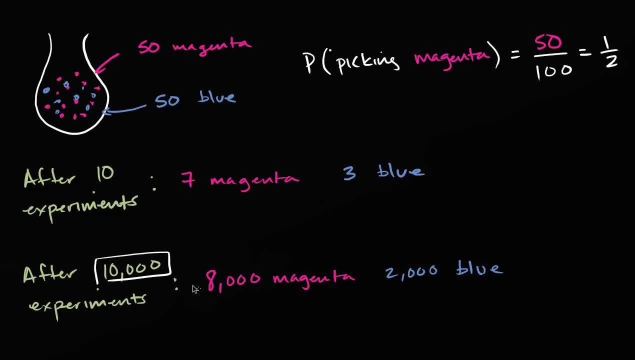 But it's not. it's very unlikely that you would have gotten this result with this many experiments, this many trials. if the true probability is 1 half, Here your experimental probability, your experimental probability is showing. look out of 10,000 trials. 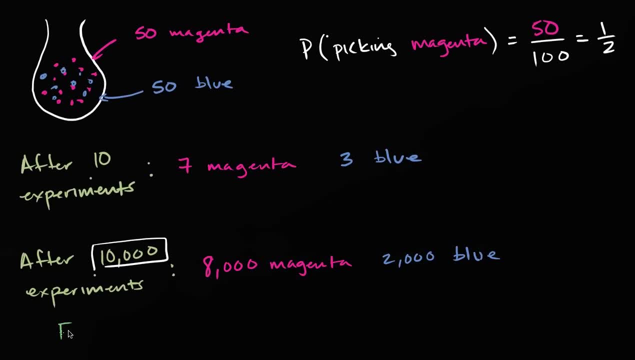 actually let me write that here: experimental probability. experimental probability here is: you had 10,000 trials or 10,000 experiments, I guess you could say, and you, and in 8,000 of them you got a magenta marble. 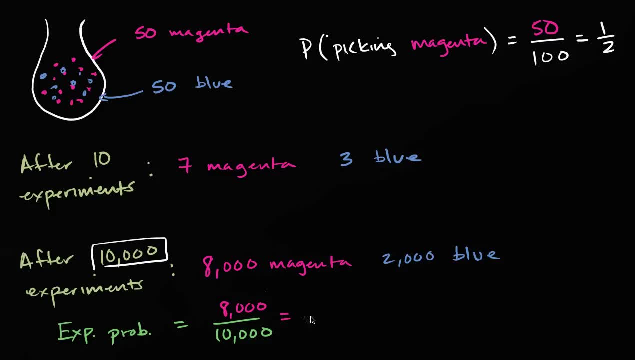 And so this is going to be 80%, or 8 tenths, So 80%. So there seems to be a difference here, And the reason why I would take this more seriously is that you had a lot of trials here. You did this 10,000 times. 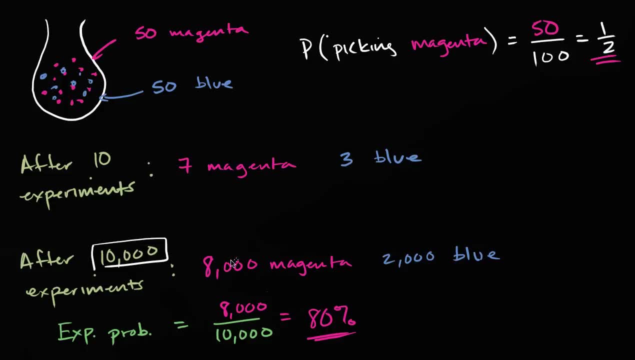 If the true probability was 1 half, it's very low likelihood that you would have gotten this many magenta. So when you think about it, you're like: look, what did I? what's going on here? What are possible explanations for this? 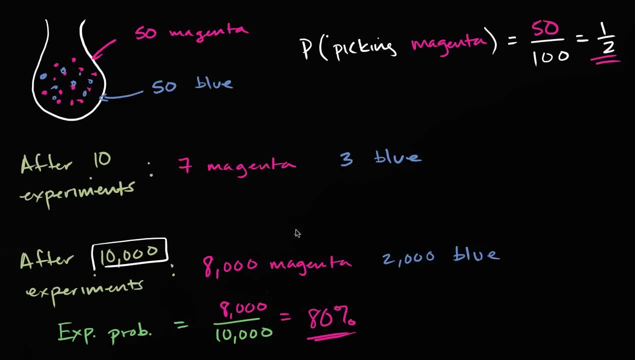 This I wouldn't have fretted about. After 10 experiments, not a big deal, But after 10,000, this would have caused me pause. You say: well, why would this happen? I mixed up the bag every time. 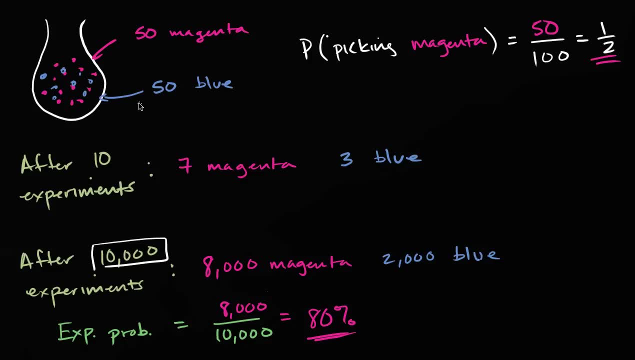 And there are some different possibilities. Maybe the blue marbles are slightly heavier And so when you shake the bag up enough, the blue marbles settle to the bottom and you're more likely to pick a magenta marble. Maybe the blue marbles have a slightly different texture.